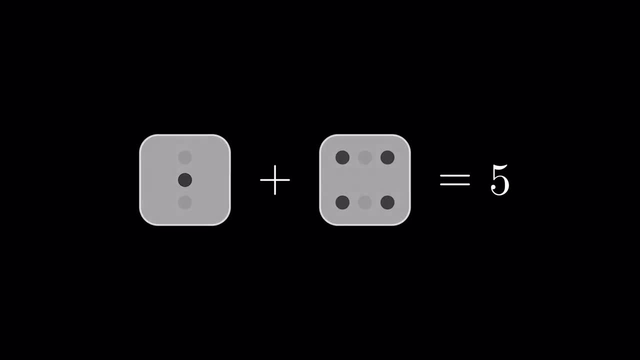 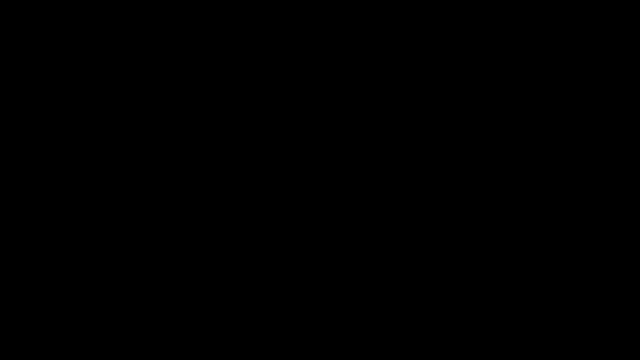 And we wonder how valuable is this information? But, as with the case of the dice, the answer changes for different values of the total energy. To dive deeper into this fact, we'll consider the case of a very simple particle for which only two states of energy are allowed. The particle which I'll show with the circle. 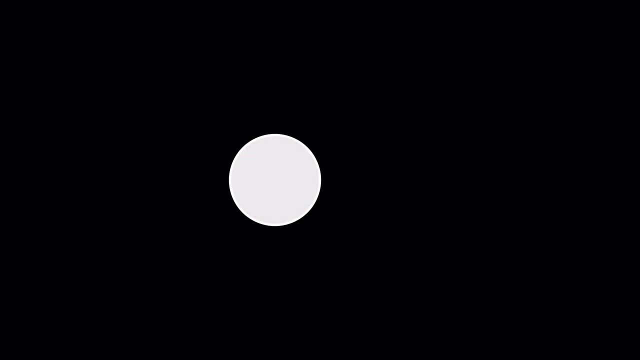 can either have energy one or zero. We want to consider a system of n of these particles, for example seven. We can choose a value for the total energy of the system- Let's say 3, without knowing how this energy is distributed among the n particles. 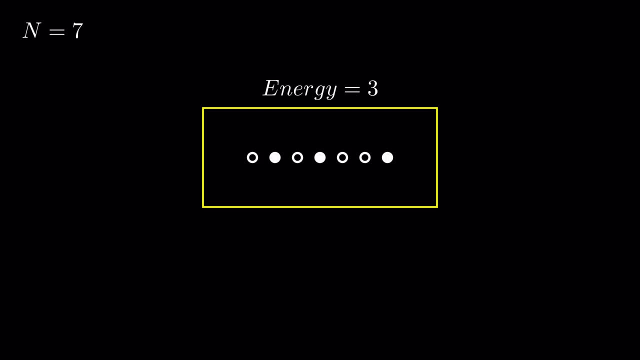 If we isolate the system, the state of the particles can change as they interact with each other, but the total energy of the system will remain constant. In our case, there could be many possible configurations of particles, But how many exactly? With energy equal to 3, we need to choose 3 particles to fill. 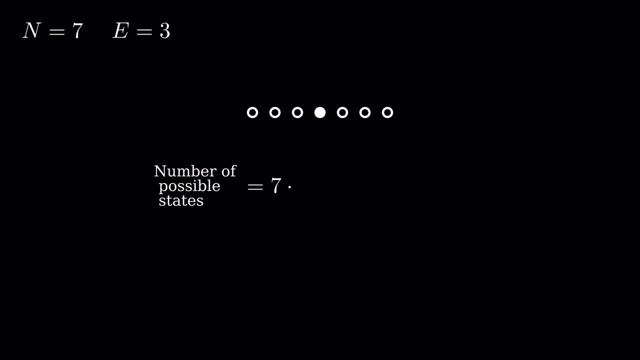 We have 7 possible choices for the first one, 6 for the second and 5 for the third. But our particles are identical and that means that if we number the 3 white particles, all the permutations of them will have to count as one unique state. 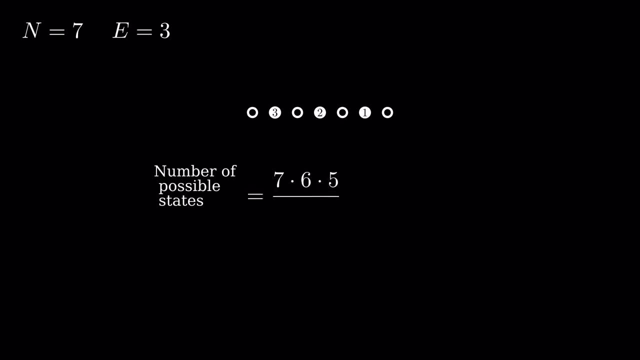 So we divide by the possible ways of combining the 3 particles, Which again is 3 choices for the first, 2 for the second and 1 for the third. You might recognize the denominator as the factorial 3, and we can also write the numerator. 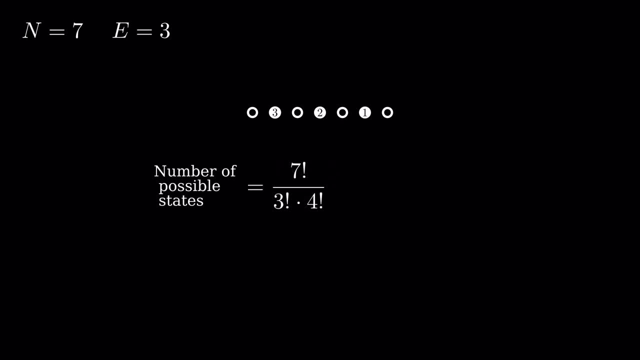 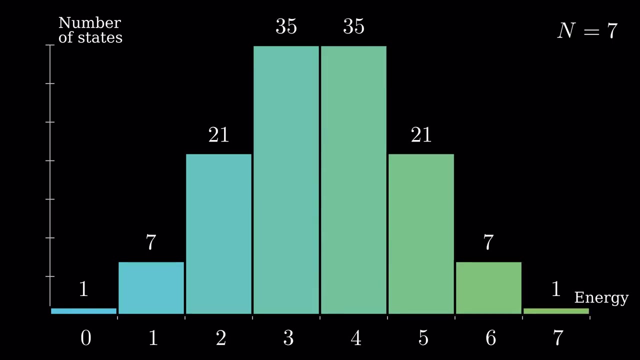 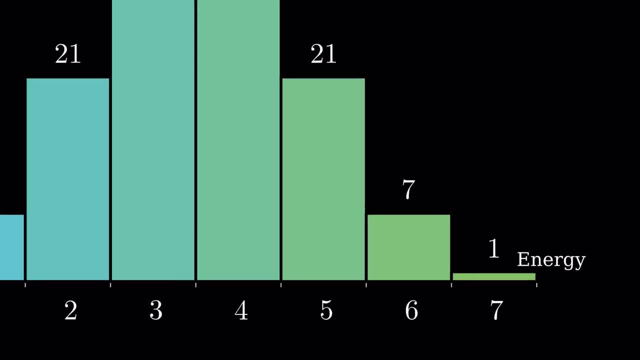 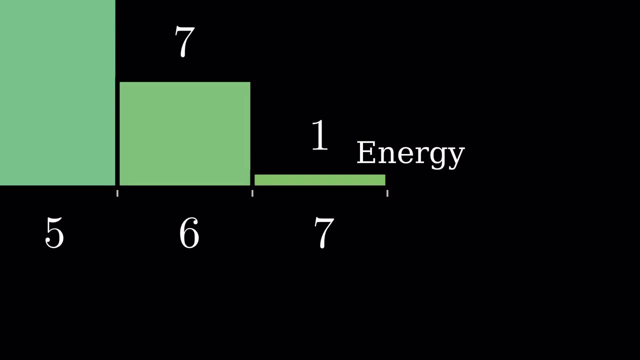 For the case of seven particles and a total energy of 7,, there is only one possible way of distributing the energy in the system so that we have no uncertainty. But in general, the more configurations are possible, the less we know about the system. 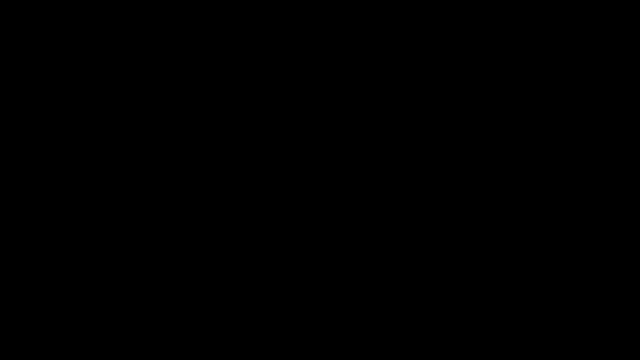 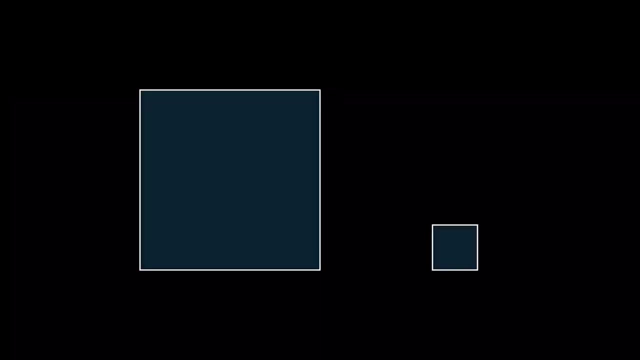 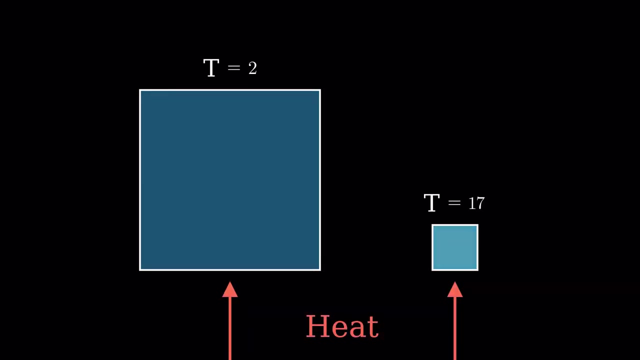 at that energy state, to relate this uncertainty to temperature. so let's think about what happens physically. Let's consider two objects of the same material, starting with the same internal energy, one much bigger than the other one If we supply the same amount of it to both objects. 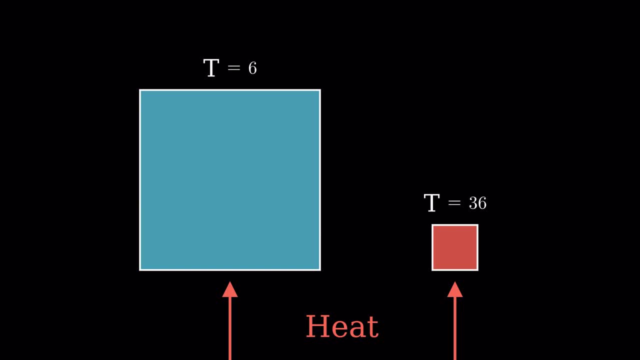 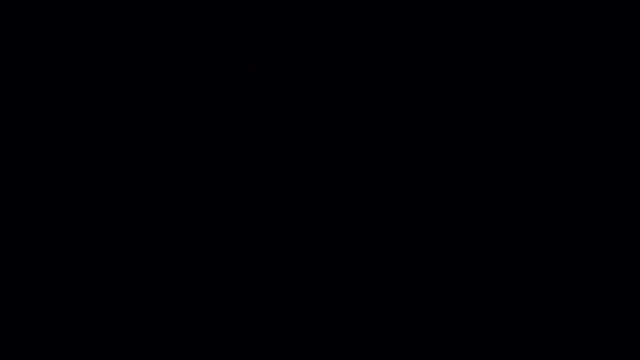 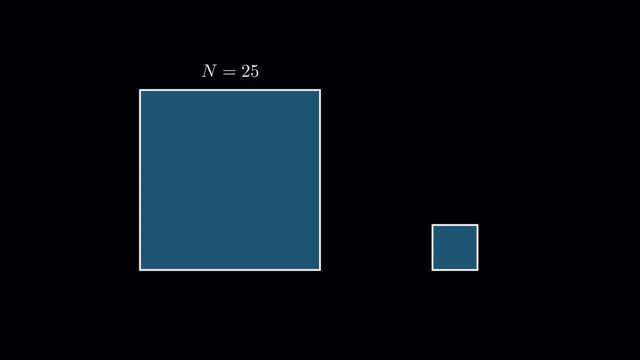 you can probably guess that the temperature of the biggest one is going to be raised less than the smaller one. Let's now consider what happens to the number of possible states. Let's say that the bigger object has 25 particles and the smaller has 4.. If we start with energy, 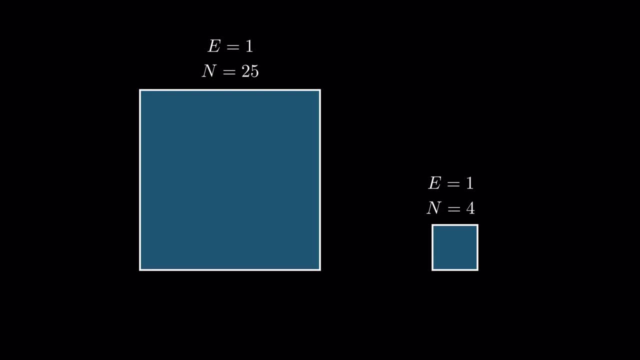 equal to 1,, we can calculate that the first system has 25 possible states and the second has 4.. For brevity, I call the number of states omega. If we supply heat, or in other words energy, to raise the total energy to 2,, the first system can now have 300 possible configurations. 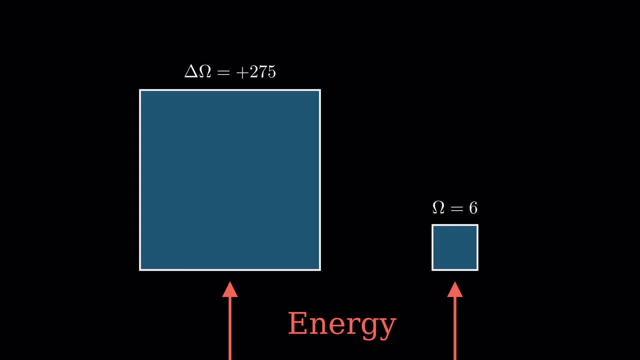 for an increase of 275,, while the second can have 6,, which increases the number only by 2.. So, to summarize, we have that the supply of energy corresponds to a smaller raise in temperature for the first system than the second, but the opposite is true for the number of possible states. 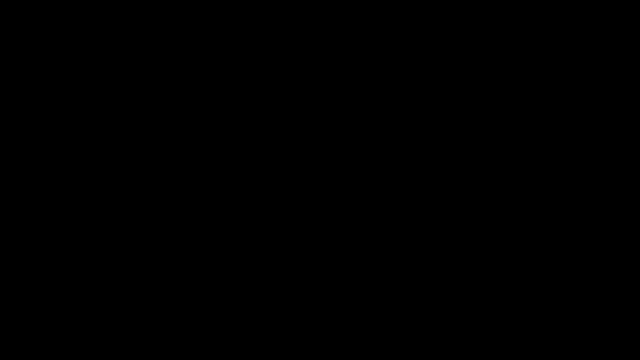 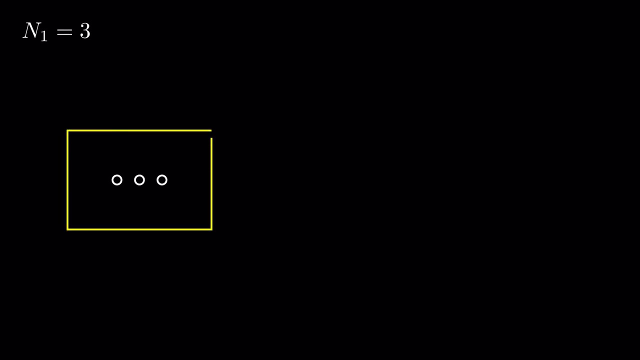 But how are the two related? Temperature is the quality that two bodies share when they are at equilibrium with each other. so let's consider the case of two systems, one with 3 particles, the other one with 4.. We'll set energy equal to 2 for the first. 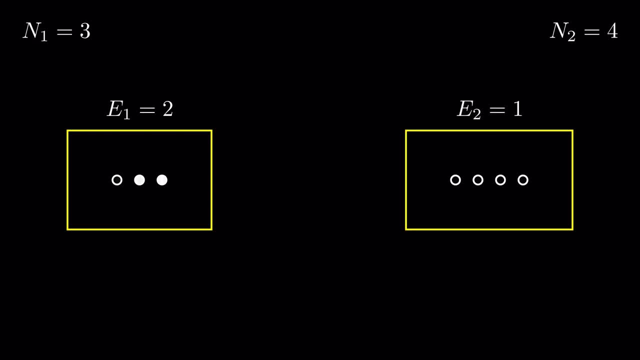 and to 1 for the second. If we put them in contact and let them exchange energy, the sum of the two energies will stay constant, but energy will flow freely from one system to the other. New configurations are possible which weren't possible before. 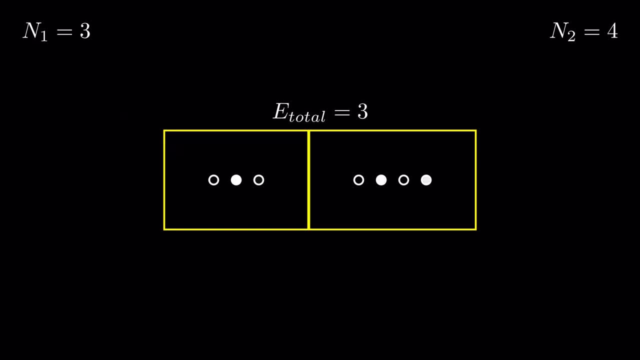 The first system might have all the energy at a certain time, or the same could be for the second system. If we fix the energy of one system to be 1, we know how to calculate the number of possible ways this could happen. The point is now to notice that the energy of the second system 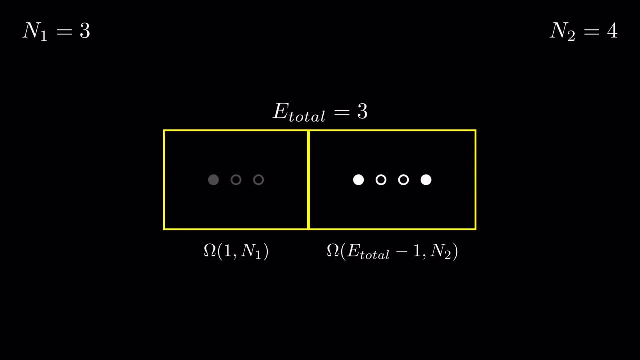 must necessarily be equal to the remaining energy, which is 2.. Or 3 minus 1.. We multiply the two numbers and since we fixed the energy of the first system at the beginning, to have the actual number of possible states we need to sum over all of the possible values for E1.. 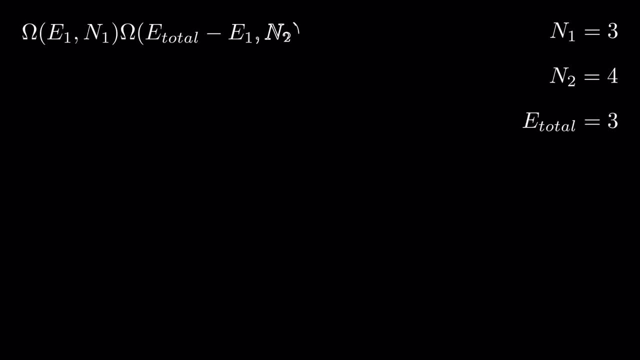 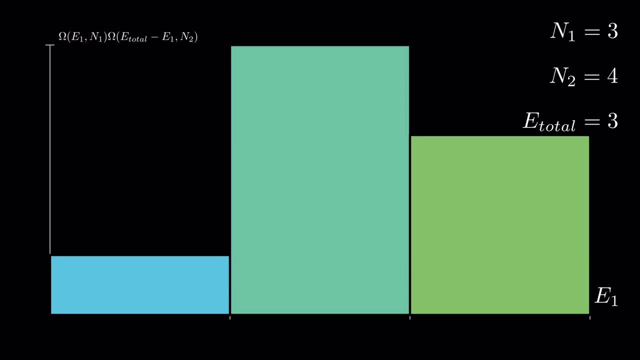 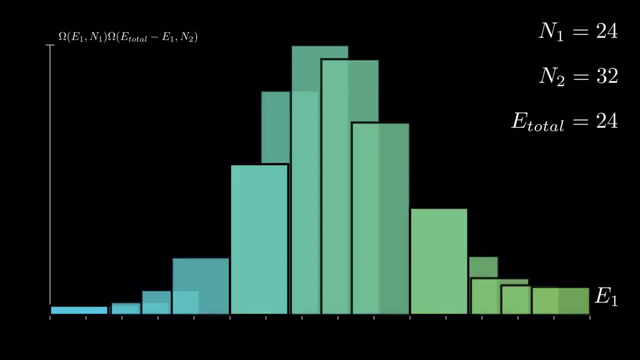 If we visualize the terms of the sum for our system, that's what they look like. Now. we are interested in systems of many particles, like the ones we encounter in everyday life, So we make the system bigger and bigger and we see what happens. 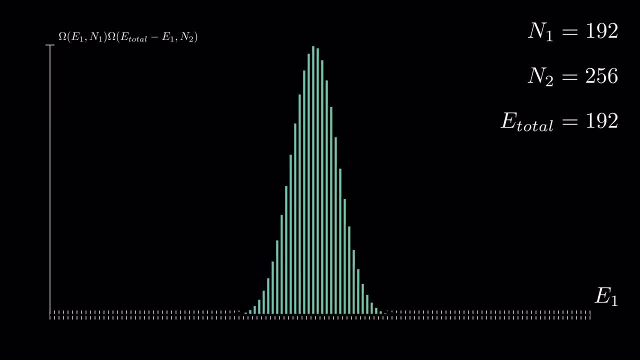 We see that the sum concentrates around the value, the equilibrium state, which also corresponds to the maximum term of the sum, or, in other words, the most probable. From now on, the sum of the two systems will be equal to the maximum term of the sum, or, in other words, the most probable. 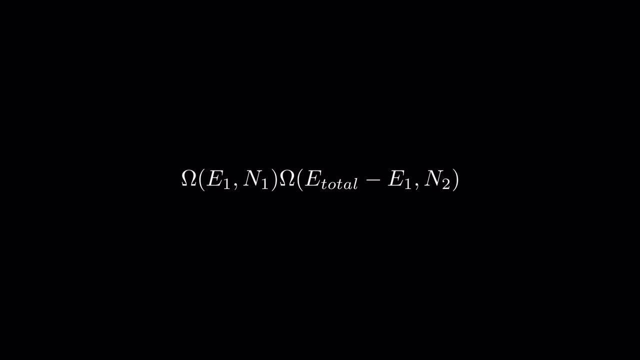 From now on, I will simplify the term of the sum by calling the first part omega1 and the second omega2.. To find the maximum of this product, we set its derivative equal to zero. This equals the derivative of the first term times the second. 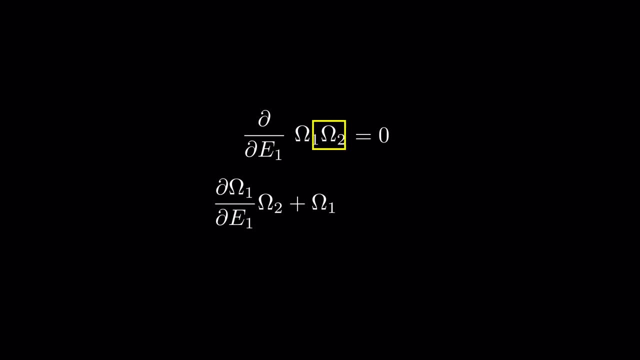 plus the first term times the derivative of the second. We then use the chain rule of derivative And the fact that the change in E2 is the same as the change in E1, but in the opposite direction, because energy must be conserved. 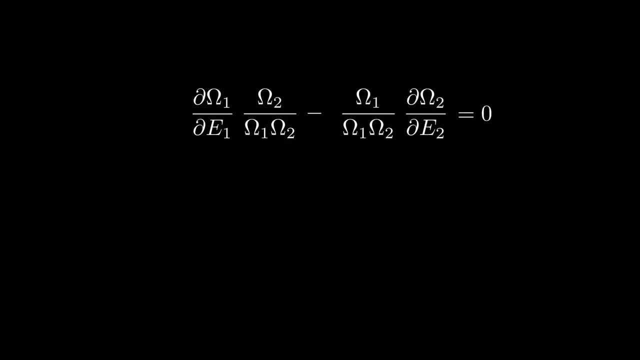 We now divide everything by omega1 times omega2.. We simplify and we move the negative term to the second member of the equation. We also include the 1 over omega into the derivative as a natural log. This quantity must be the same for the two systems.